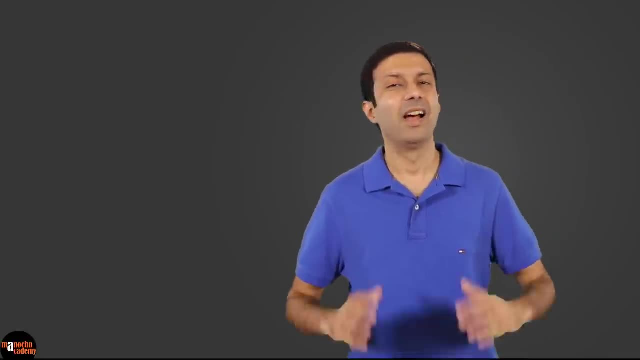 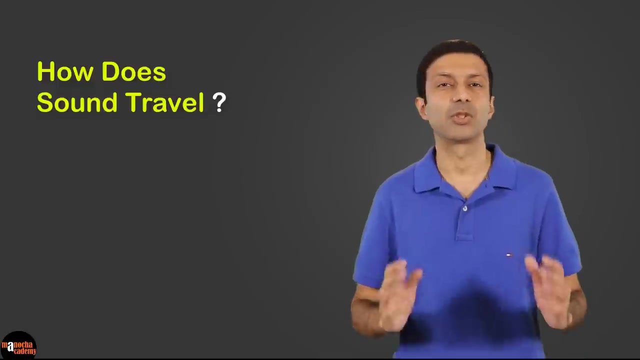 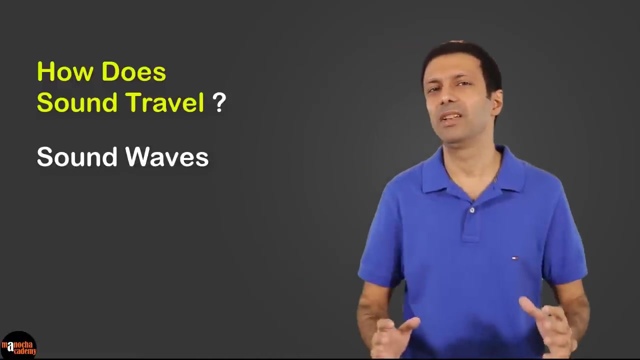 Hello, hello, can you hear me? Hi friends, have you ever wondered how is this sound travelling to your ears? That's what we are going to explore in this video. I'm going to make the concept of sound waves really simple and easy for you. 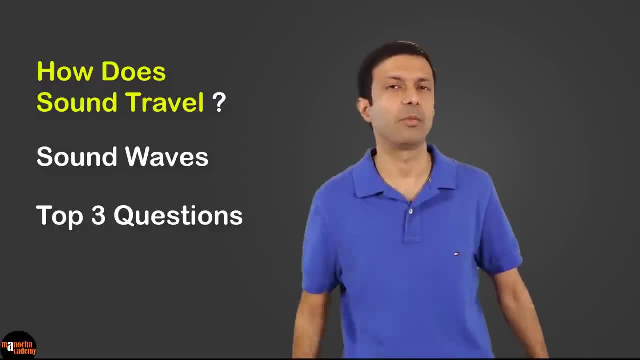 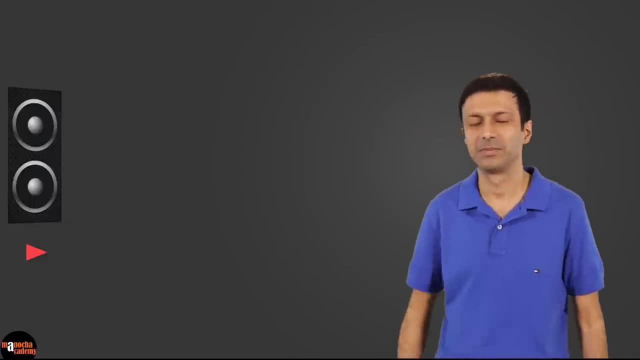 And then we'll finish off with our top three exam-oriented questions on this topic. Let's say you're relaxing and listening to music from your music system. The question we are looking at is: how is the sound from the speaker travelling to your ear? 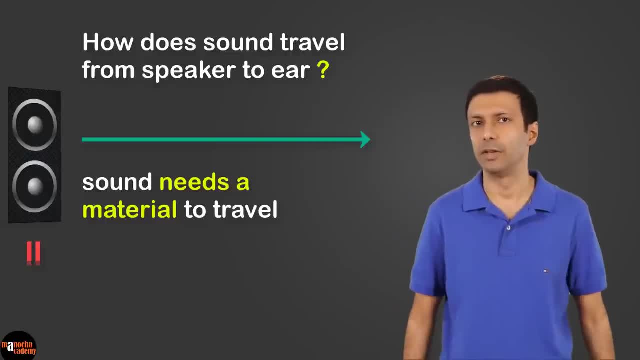 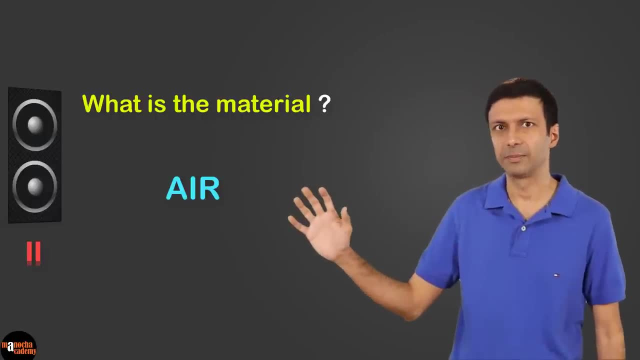 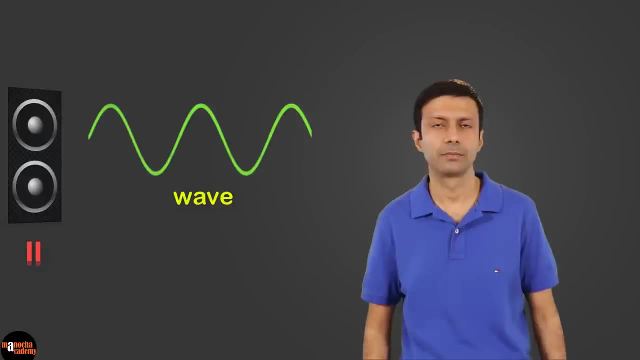 Sound is a form of energy that needs a material to travel. So what do you think is the material? in this case, The material is air. Sound is travelling as a wave or a disturbance of the air particles. Now, what do we mean by the term wave? 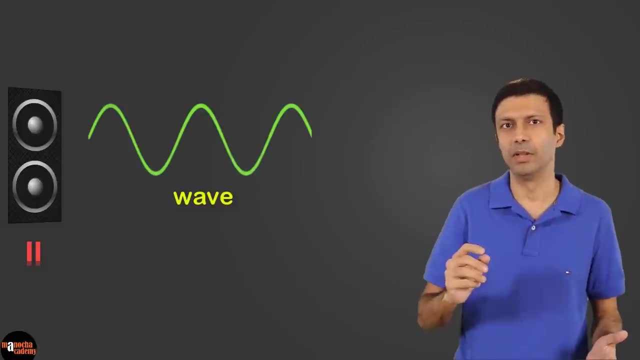 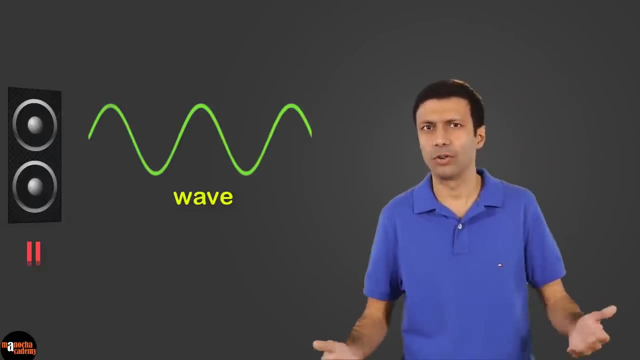 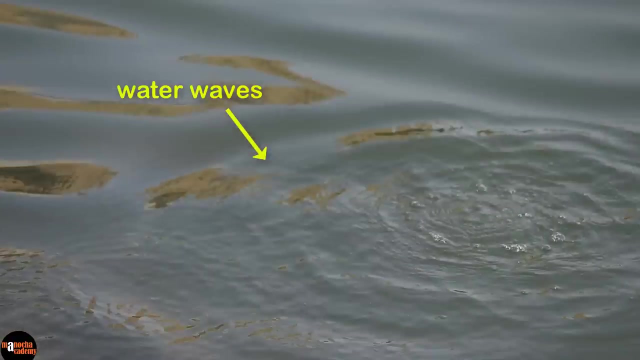 Since the air particles are invisible. so let's take the example of water. I'm sure you've thrown a pebble in a pond or a lake, right? So before you throw the pebble, the water is still, And once the pebble falls in, you can see the waves or the ripples travelling on the surface of water. 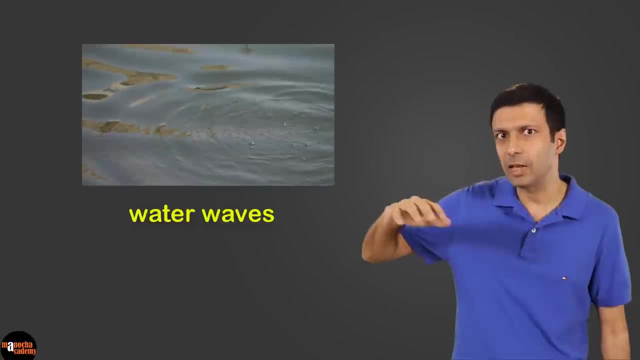 Similarly, sound waves can also travel on the surface of water. Similarly, sound waves can also travel on the surface of water. Similarly, sound is travelling as a disturbance of the air particles. Now there are some differences between a sound wave and a water wave. 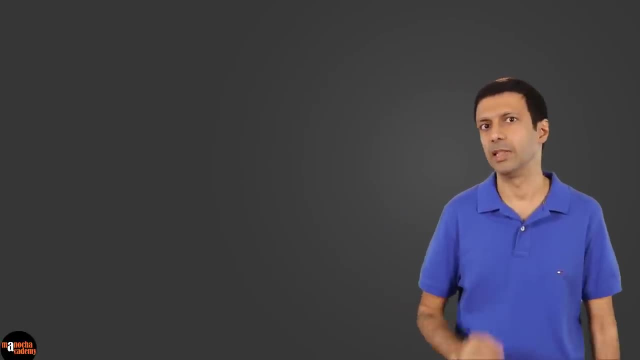 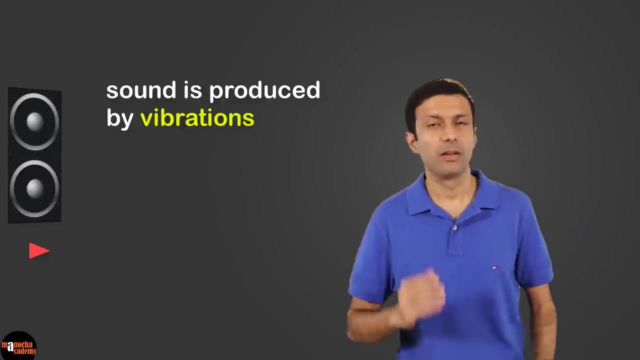 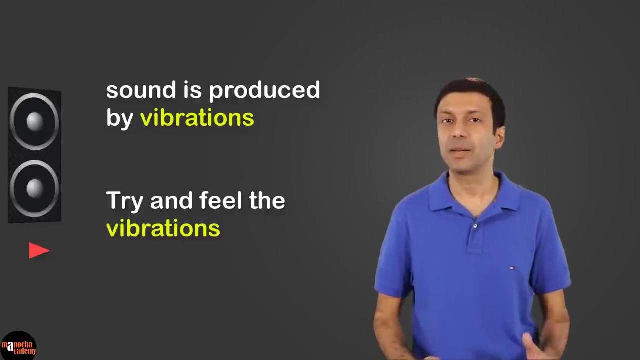 But we are not going to go into the details in this video. Now, when the music is playing, the speaker is vibrating, Because sound is produced by vibrations. If you don't believe me, why don't you try it yourself? Next time your music system is on, you can put your hand on the speaker. 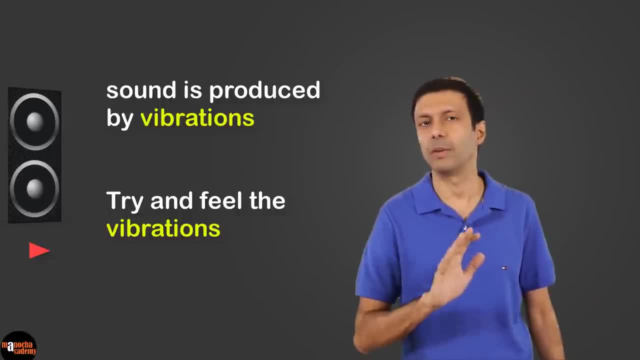 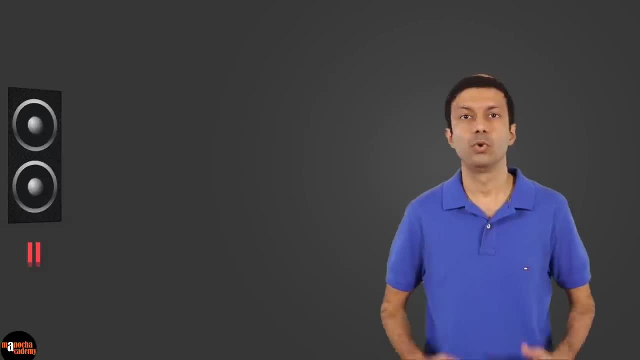 Next time your music system is on, you can put your hand on the speaker. Next time your music system is on, you can put your hand on the speaker And go ahead and feel the vibrations. I'm sure you can feel it, especially if the music is a bit loud. 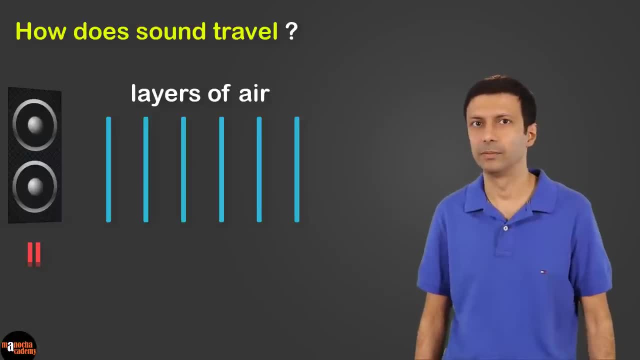 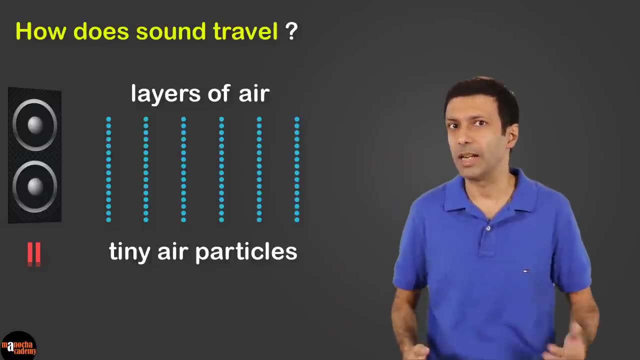 To understand how sound travels, I've gone ahead and drawn the layers of air here. To understand how sound travels, I've gone ahead and drawn the layers of air here. Each layer of air is made up of tiny, tiny air particles, So you can imagine this series or layers of air between the speaker and yourself. 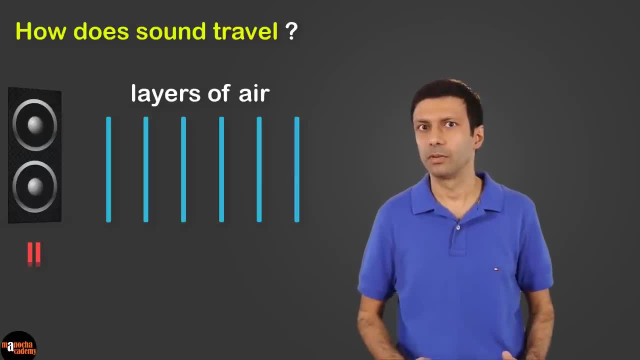 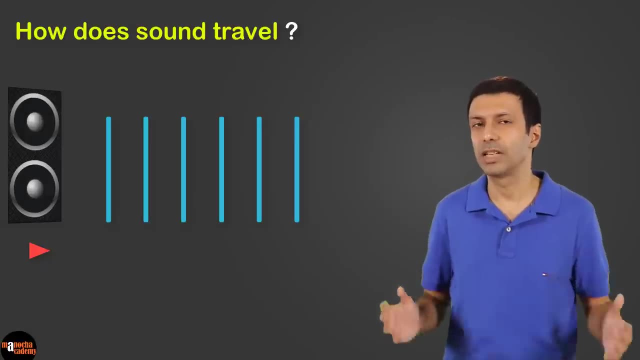 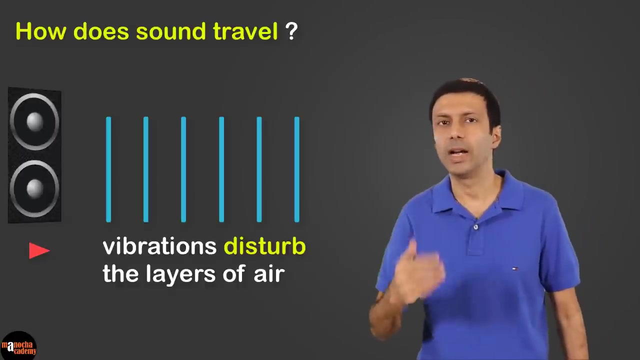 So you can imagine this series or layers of air between the speaker and yourself. music is off, these layers are stationary, that is, they are not moving. now imagine the music is on, so vibrations are coming out of that speaker, and these vibrations will go ahead and disturb the layers of air, so the vibrations will go. 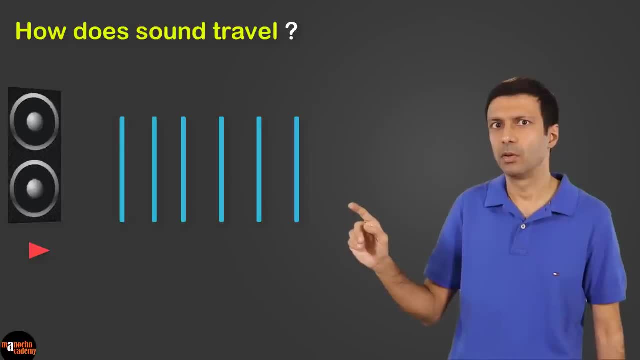 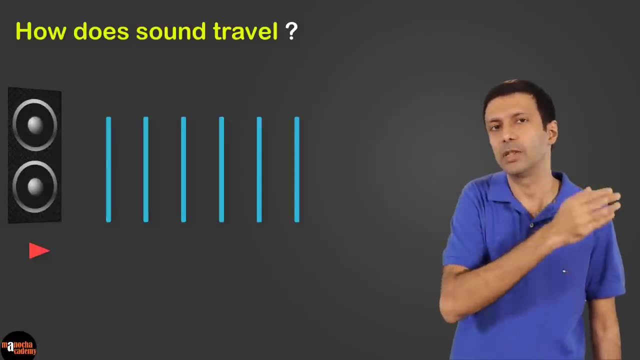 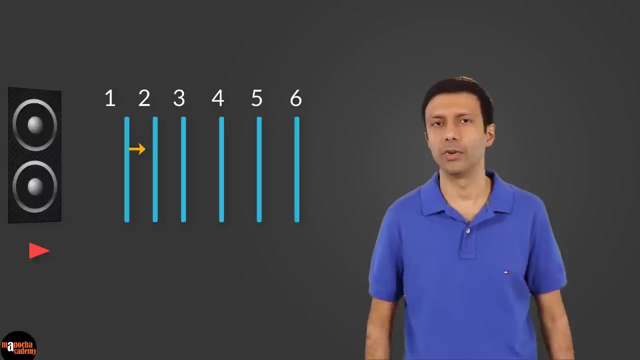 ahead and disturb the first layer of air, which goes ahead and disturbs the second layer of air, and this disturbance will continue through the layers of air. now, if you consider the first layer of air here, that will go ahead and push the second layer of air, but because air is an elastic medium, which means it has 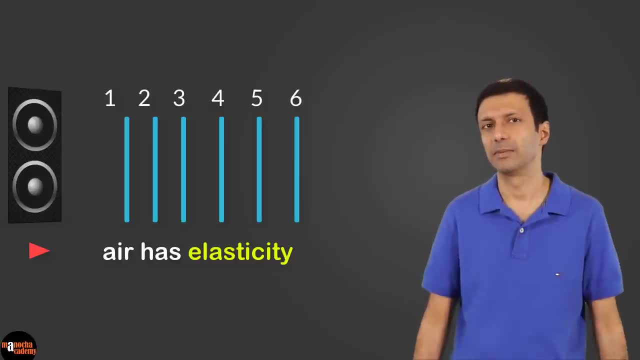 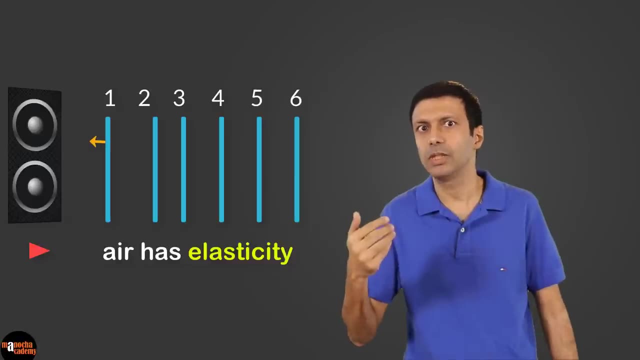 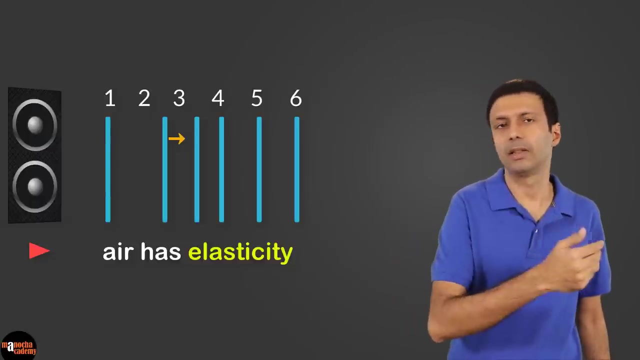 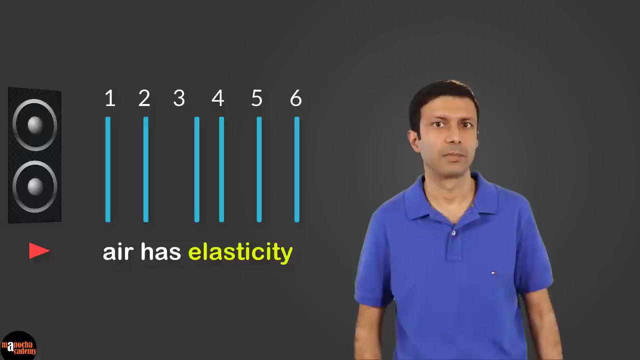 some elasticity it behaves like a rubber band. so the first layer, after disturbing the second layer, will go ahead and spring back to its original position. you, similarly, the second layer of air, after disturbing the third layer, will spring back to its original position due to the elasticity of air and this process. 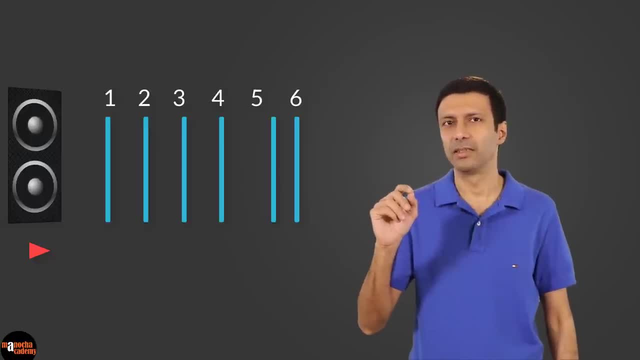 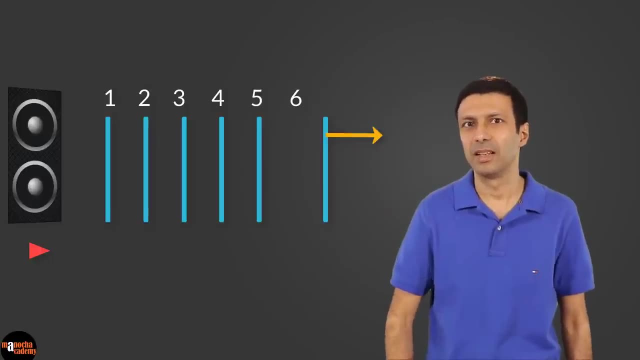 continues. if you look at the final layers of air, they will push each other and then that last layer of air goes and hits my ear. that disturbance goes and vibrates the eardrum in my ear, which causes the sensation that the допughn is now saved and then it internally makes its 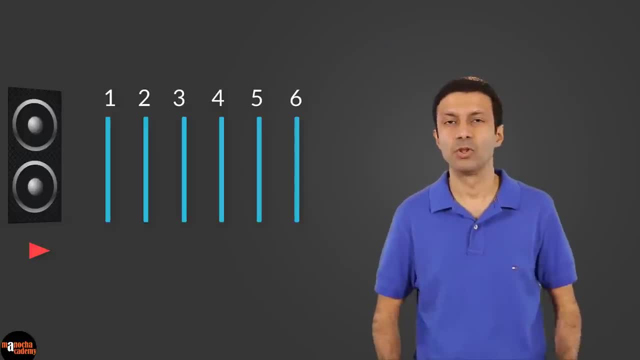 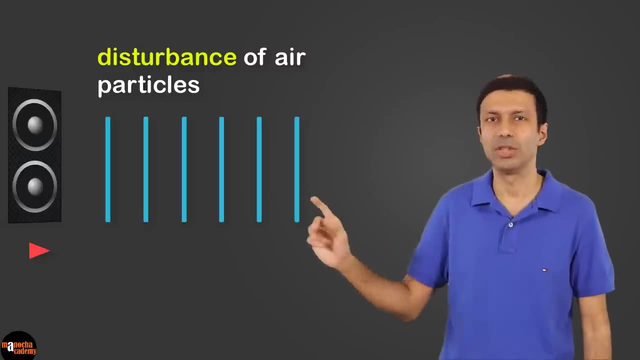 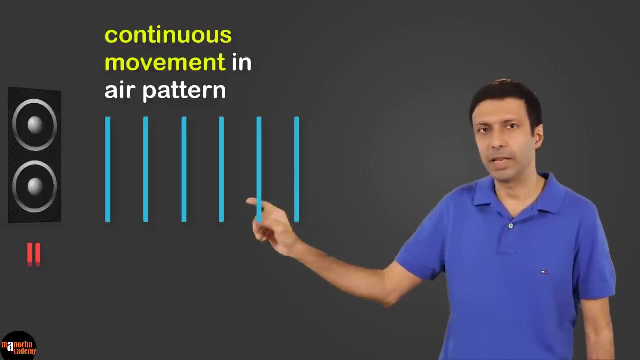 of listening or hearing, so sound is traveling as a disturbance of the air particles. that's how we can listen to the music playing. so as the music keeps playing, vibrations are coming out of that speaker continuously. this causes a continuous movement or disturbance in the air pattern between the speaker and the listener. now what would this air pattern look like? 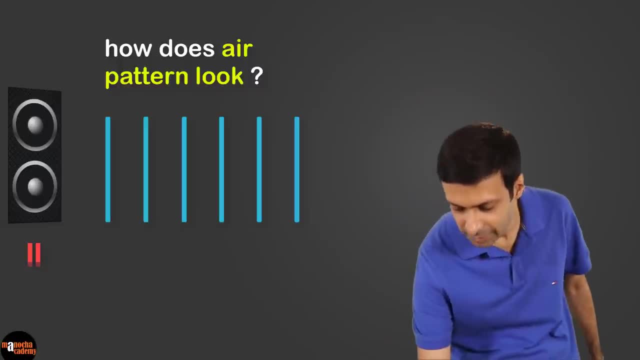 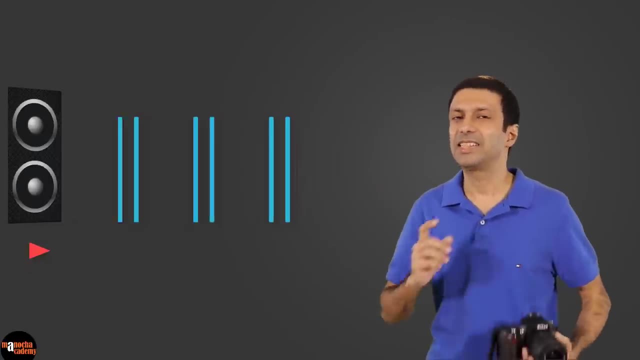 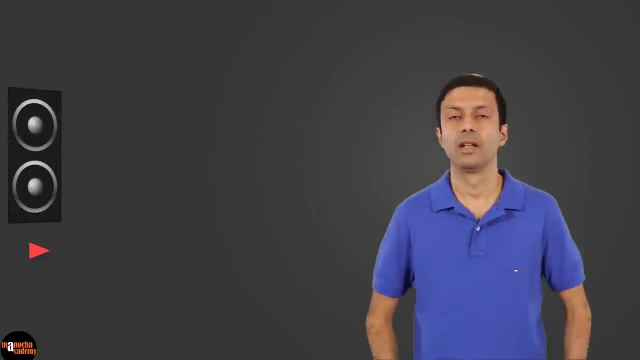 let me help you visualize this. so let's turn on that music one more time and let's look at the air pattern. now, as the music is playing, let's take a snapshot of the layers of air. here's a photo of the layers of air that we just clicked. 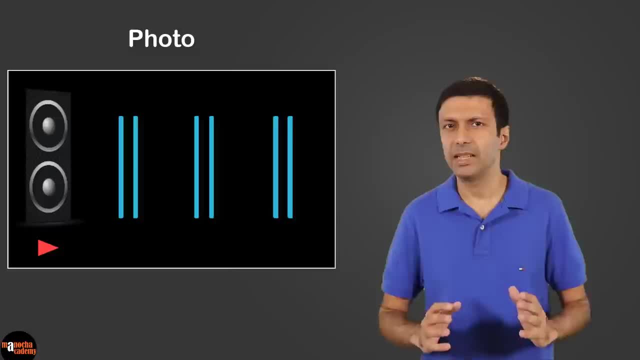 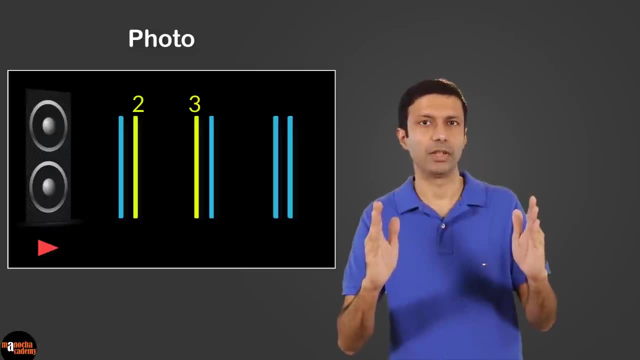 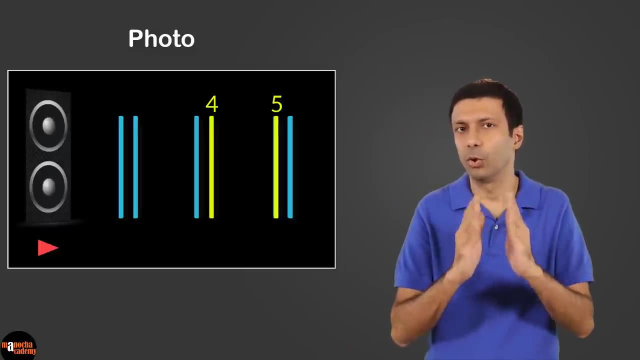 if you look closely at the pattern here, you can see that the first two layers are close to each other. the second and the third layer are far from each other. the third and the fourth are again close to each other. the fourth and the fifth are far from each. 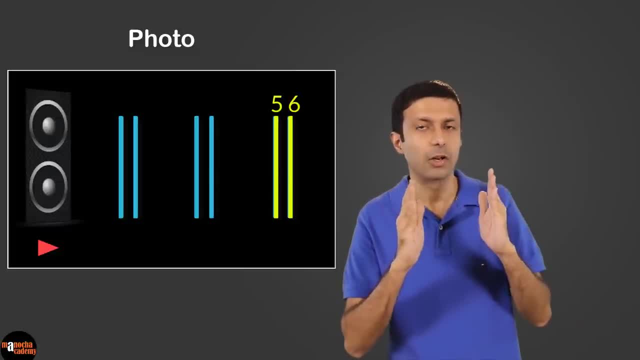 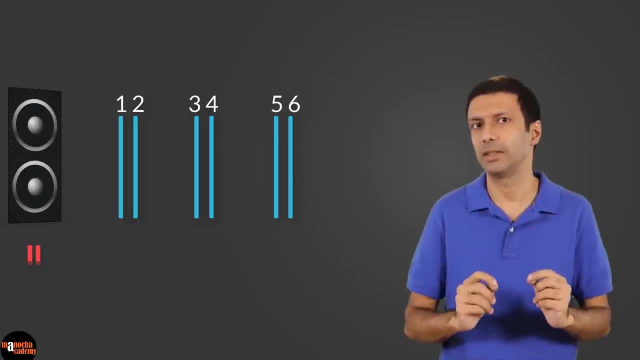 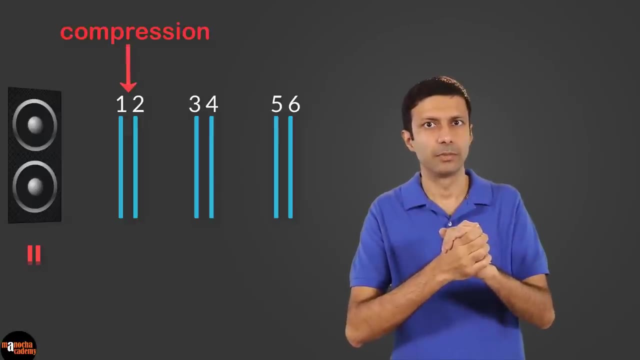 other. the fifth and the sixth are close to each other, and so this pattern continues. and can you notice the alternating pattern here? when the two layers of air are close to each other, it's called a compression, and when the two layers of air are far from each other, it's called a rare refraction. 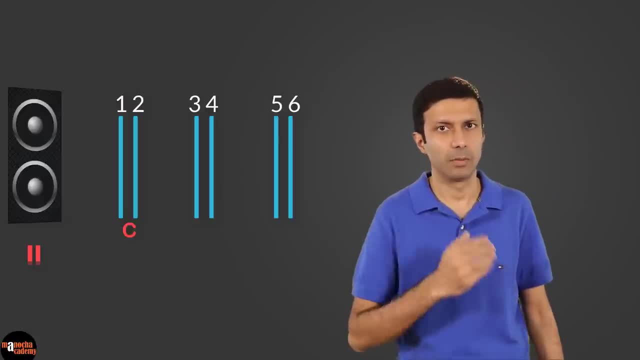 and, as you can see, there's an alternating pattern of compression, rare refraction, compression, rare refraction and so on. a compression is a region of high pressure- because you can see that i'm pressing my hands here- and rare refraction is a region of low pressure. 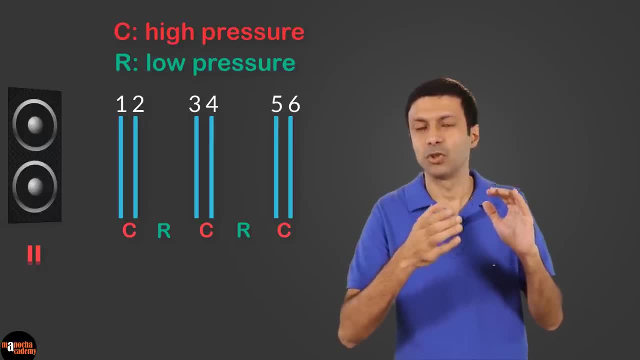 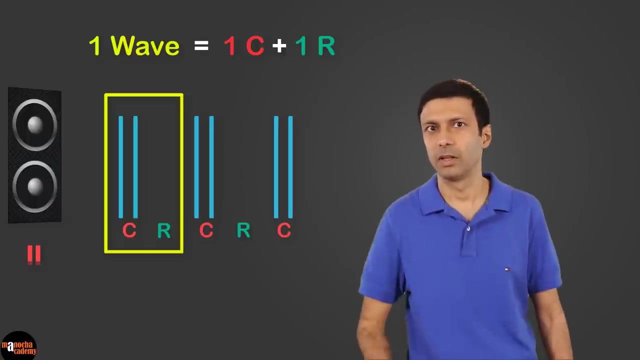 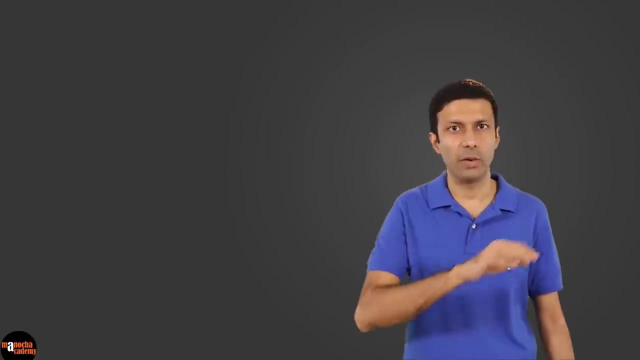 so that's when i release my hand. so, once again, compression is high pressure and rare refraction is low pressure. one wave is defined as one compression and one rare refraction, or a region of high pressure and low pressure. i'm sure you've seen this wave-like pattern in your textbooks. right, it looks like these hills and 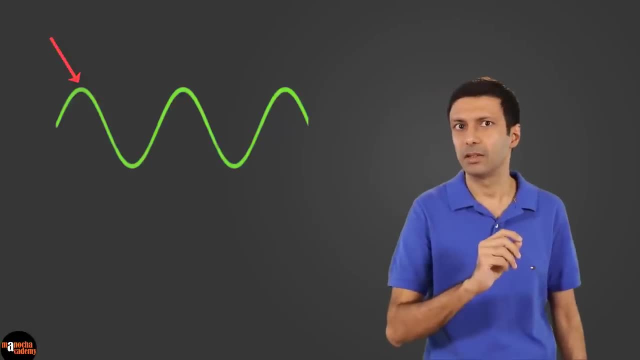 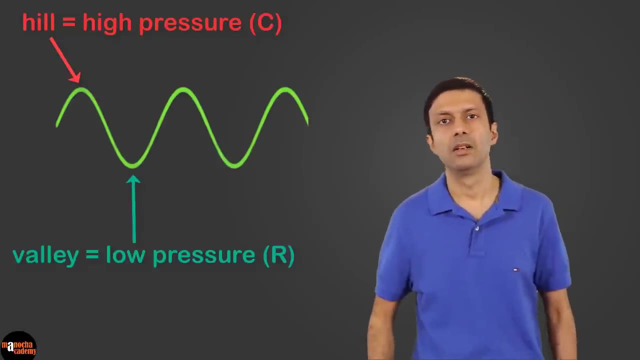 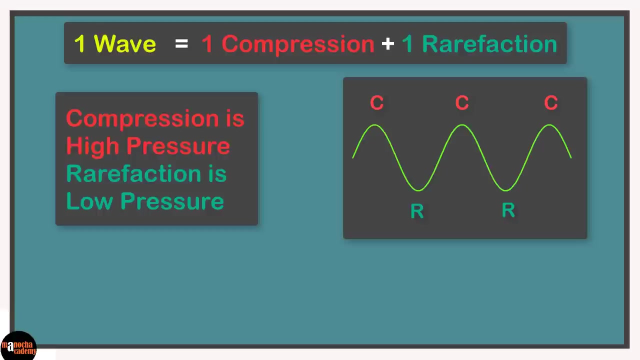 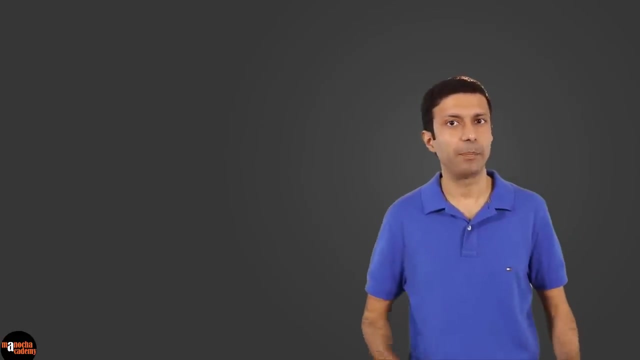 valleys. the hill represents a region of high pressure, so that's the compression, and the valley represents a region of low pressure, so that's the rare refraction. let's pin the definition of wave, compression and rare refraction on our concept board. now let's see if we can depict this wave. 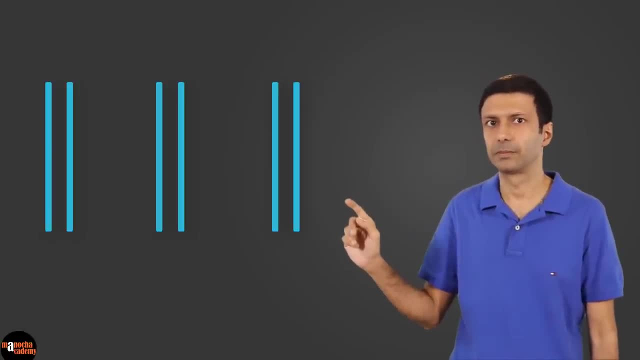 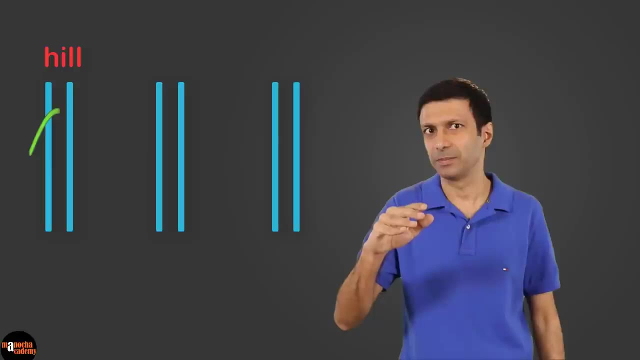 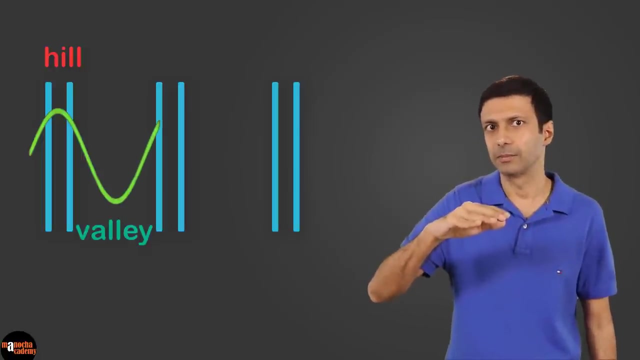 like diagram on our layers of air here. so the first two layers, they form a compression, so that's our hill right now. the next two layers, they form the rare refraction, so that's our valley, and then again there's a hill which is followed by a valley. so can you see this alternating? 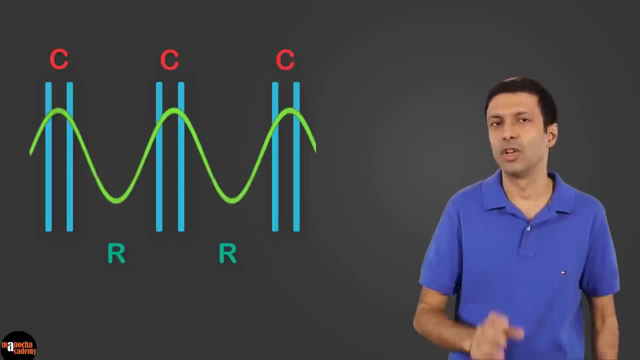 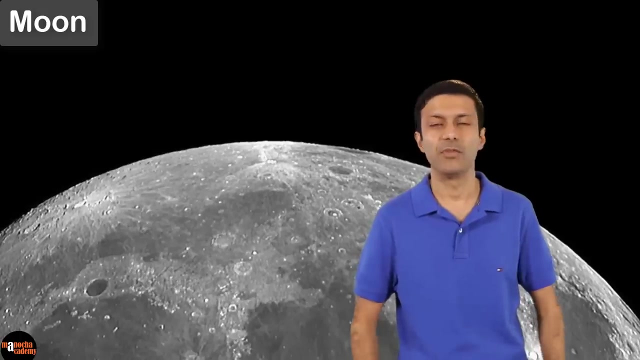 compression and rare refraction pattern here. so that's the connection between the wave-like diagram that you see in your textbooks and the layers of air through which sound is traveling. now let's imagine you and i are on the moon and we are having a discussion about sound waves. 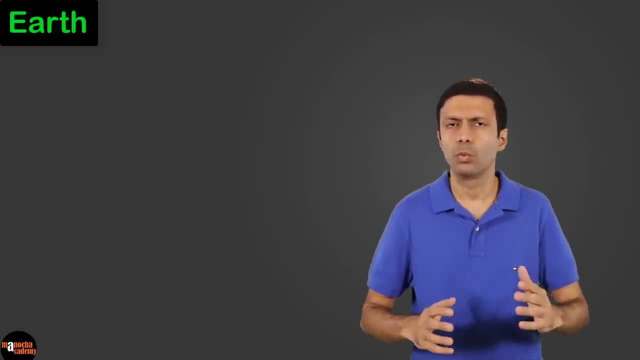 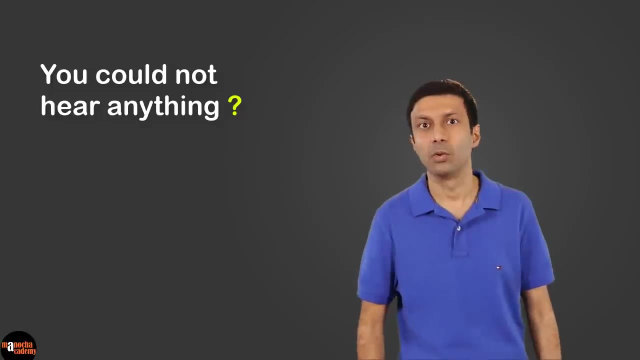 now let's say we are back to the earth. so why are you looking so confused? you couldn't hear what i said. that's right. we can't hear on the moon because there's no air or atmosphere on the moon. sound needs air to travel and that's why you can't have this conversation. 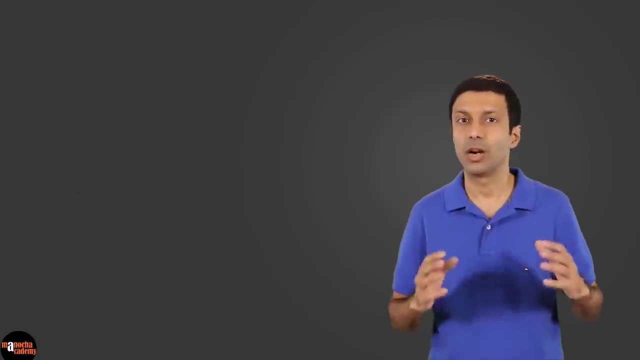 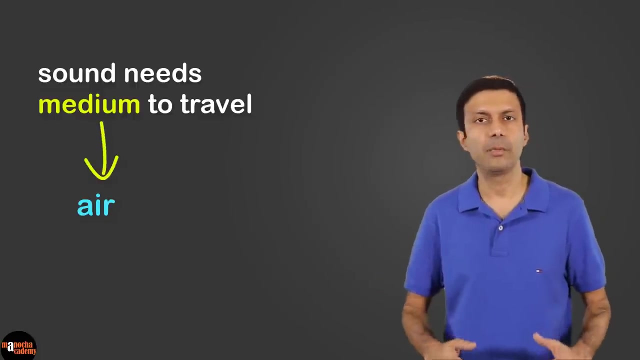 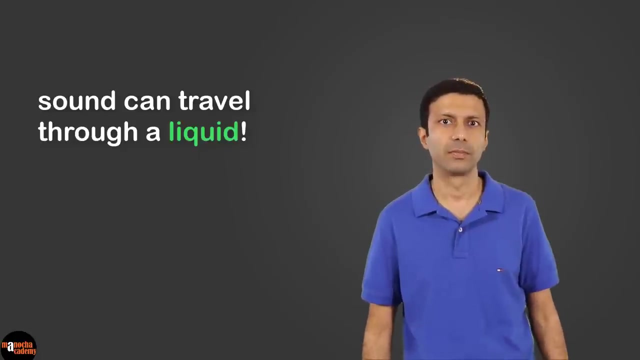 that we are having here on the moon. so sound needs a material medium to travel, and the material can be air-like here, or it can even be a liquid. so the material can be air-like or it can even be a liquid, such as water. yes, sound can travel through a liquid. i actually experienced this at my 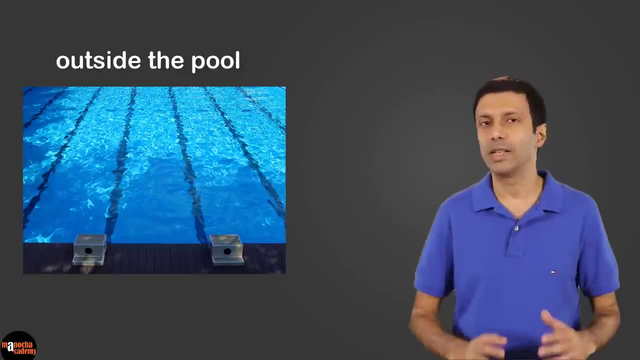 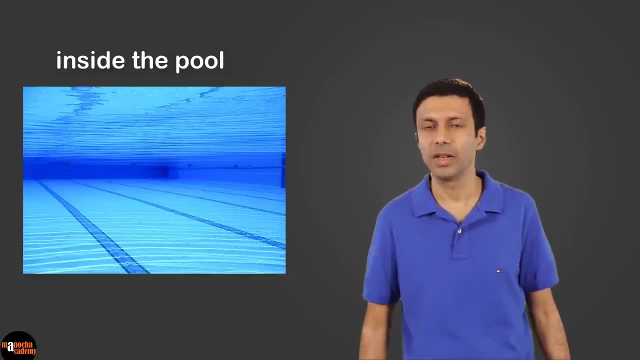 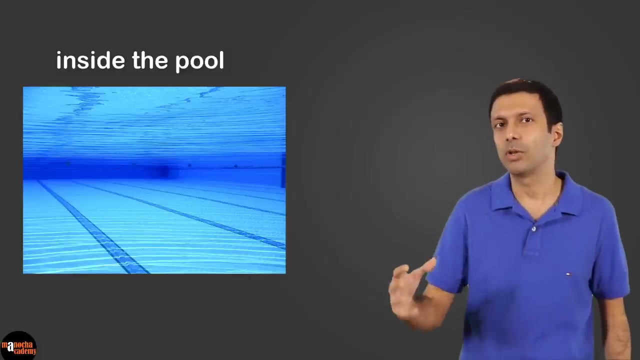 university many years back. so one day when i went swimming i couldn't hear any music outside, but the moment i entered the pool and started swimming, i could clearly hear music. then i realized that they've actually got an underwater music system, so speakers are installed under the surface of water, and it was such an amazing experience that, even after so many years, 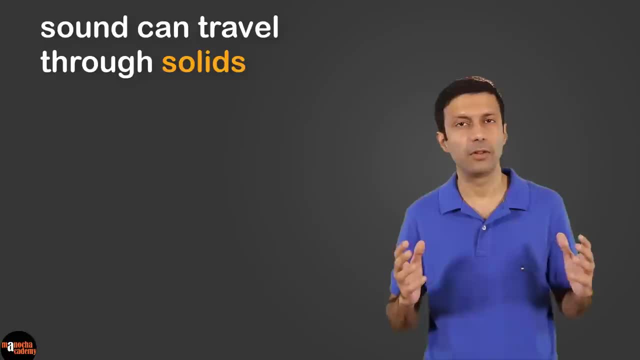 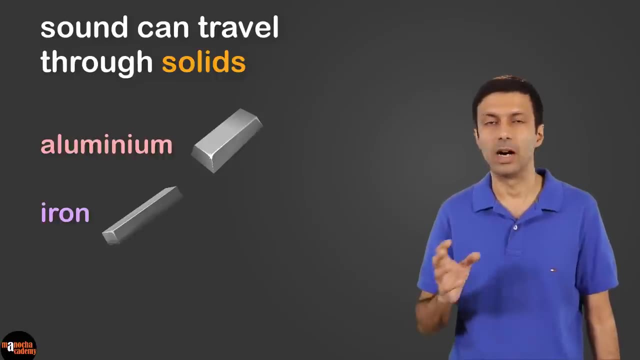 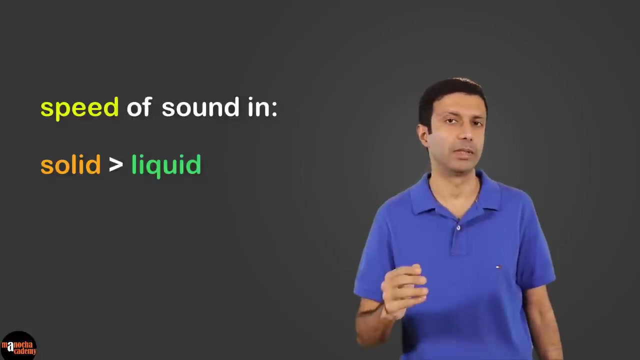 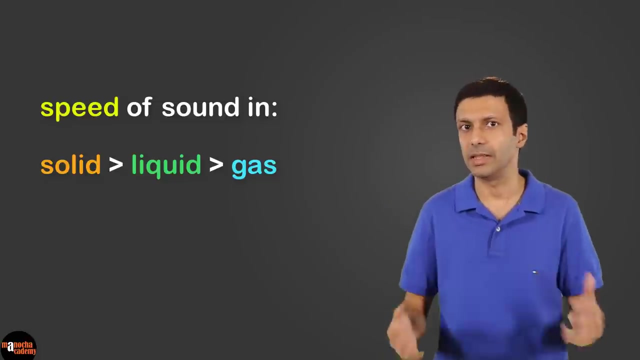 i still remember it. sound can even travel through solids like metals. for example, sound can travel through aluminium, iron, steel. in fact, sound travels much faster in solids as compared to liquids and much faster in liquids as compared to gases. that's why in the olden days, to listen for an approaching train, they would actually put. 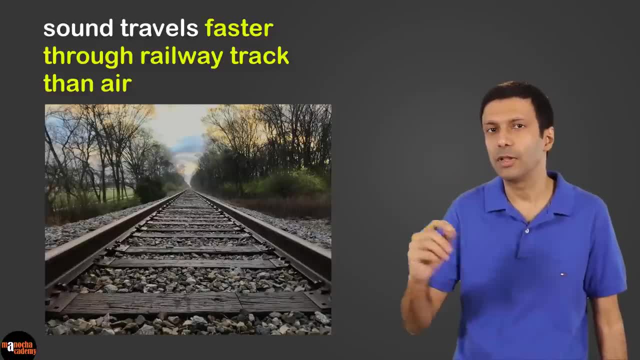 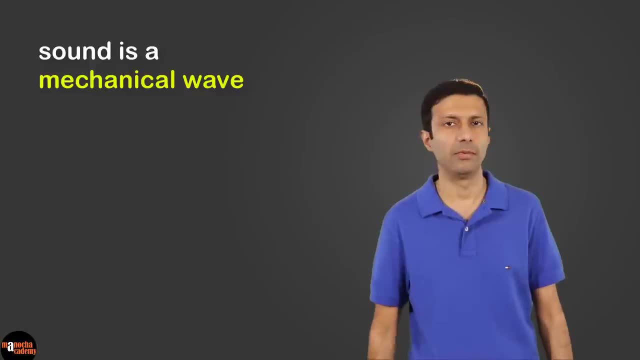 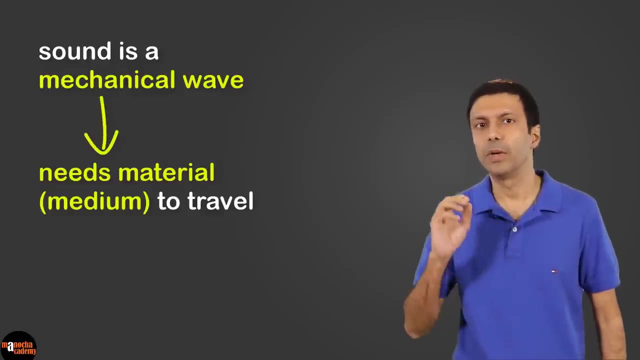 their ear on the railway track. because sound travels faster through the railway track than through air, sound is classified as a mechanical wave. now, what does this term mean? a mechanical wave is a wave that needs a material to travel, or it needs a medium to travel for sound.